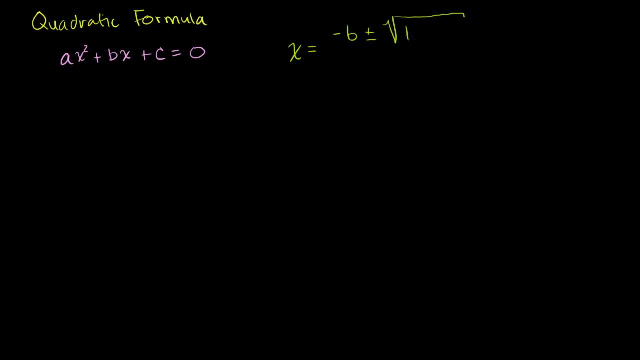 or minus the square root. So we're going to take the square root of b, squared minus 4ac, all of that over 2a And I know it seems crazy and convoluted and hard for you to memorize right now, but as you get a lot more practice you'll. 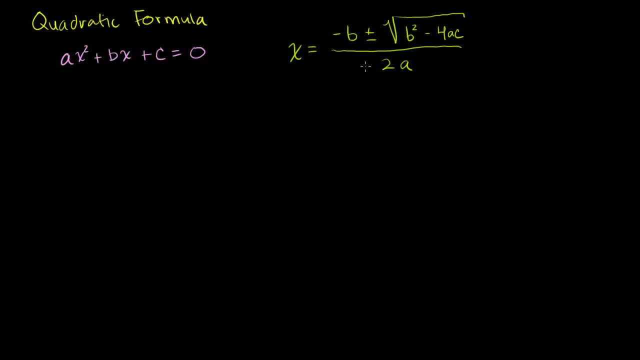 see that it actually is a pretty reasonable formula to stick in your brain someplace And you might say, gee, this is a wacky formula. Where did it come from? And in the next video I'm going to show you where it. 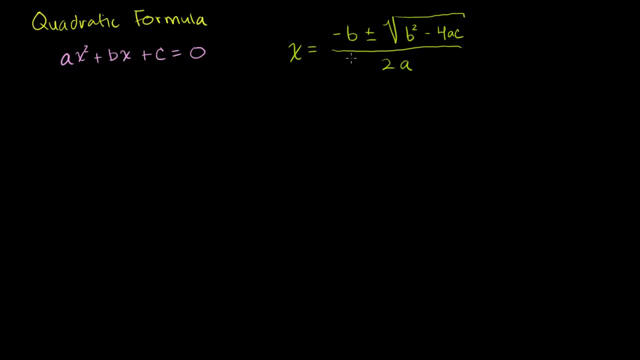 came from, but I want you to just get used to using it first. But it really just came from completing the equation. You're completing the square on this equation right there. If you complete the square here, you're actually going to get this solution. 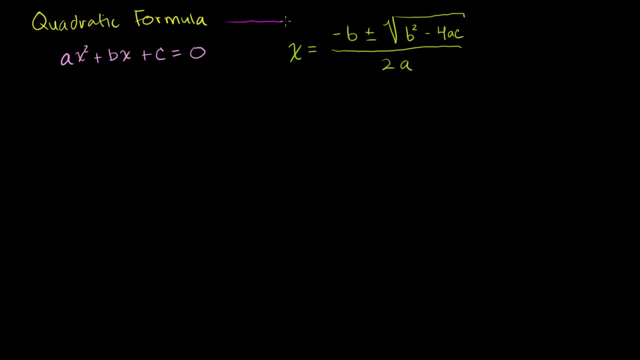 And that is the quadratic formula right there. So let's apply it to some problems. Let's start off with something that we could have factored, just to verify that it's giving us the same answer. So let's say we have x squared plus 4x minus 21 is equal to 0.. 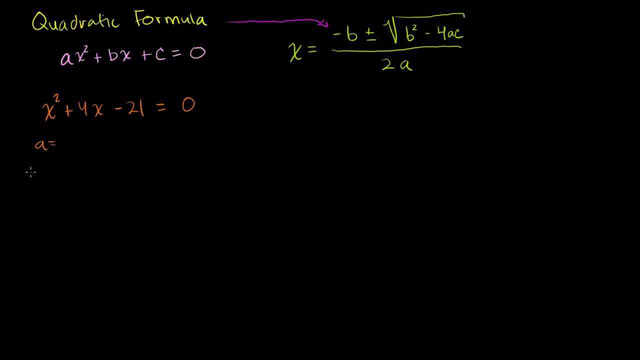 So in this situation a is equal to. let me do that in a different color. In this situation, a is equal to 1.. The coefficient on the x squared term is 1.. b is equal to 4.. b is equal to 4, the coefficient on the x term. 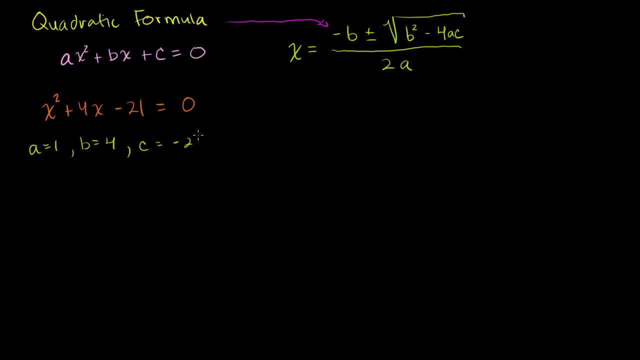 And then c is equal to negative 21,, the constant term, And let's just plug it in the formula. So what do we get? We get x. This tells us that x is going to be equal to negative b. Negative b is negative 4.. 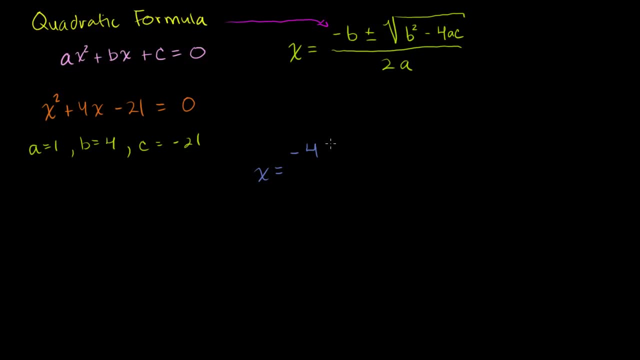 Negative 4, I put a negative sign in front of that Negative b plus or minus the square root of b squared. b squared is 16.. 4 squared is 16.. Minus 4 times a, which is 1, times c, which is negative 21.. 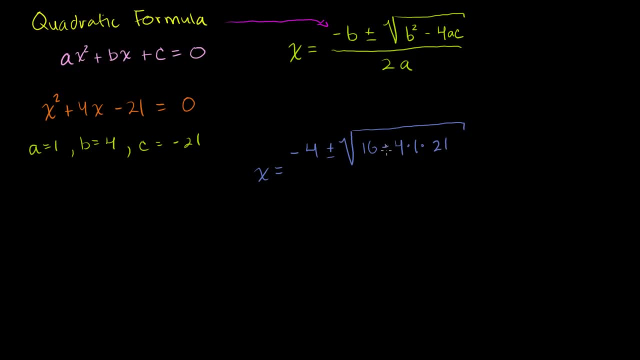 So we can put a 21 out there and that negative sign will cancel out Just like that, with that. This is the first time we're doing it, Let me not skip too many steps. So negative 21,, just so you can see how it fit in. 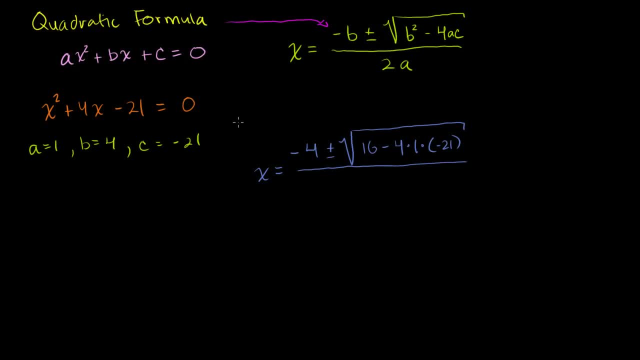 And then all of that over 2 times a, Over 2 times a, a is 1.. So all of that over 2.. So what does this simplify? or hopefully it simplifies. So we get: x is equal to negative 4 plus or minus the. 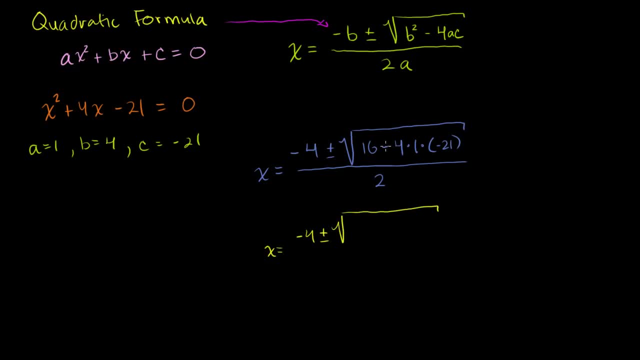 square root of see. we have a negative times a negative That's going to give us a positive, And we have 16 plus. let's see: this is 4 times 1 is 4.. Times 21 is 84.. 16 plus 84 is 100.. 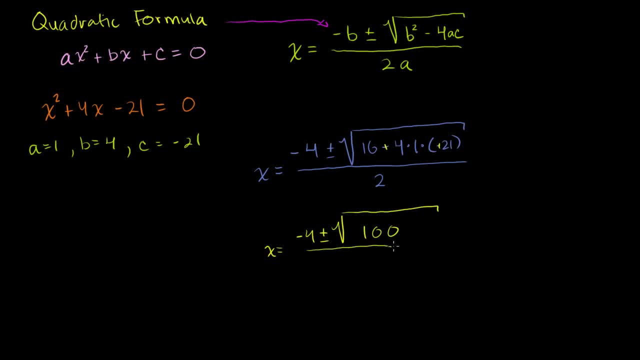 That's nice. That's a nice, perfect square. All of that over 2.. And so this is going to be equal to negative 4 plus or minus 10 over 2.. We could just divide both of these terms by 2, right now. 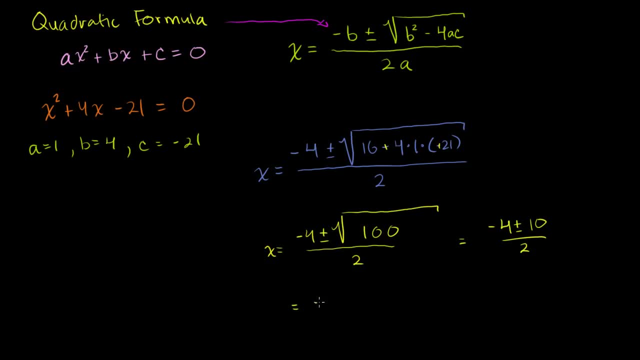 So this is equal to negative 4 divided about 20.. U divided by 2 is negative 2,. plus or minus 10 divided by 2 is 5.. So that tells us that x could be equal to negative 2 plus 5,. 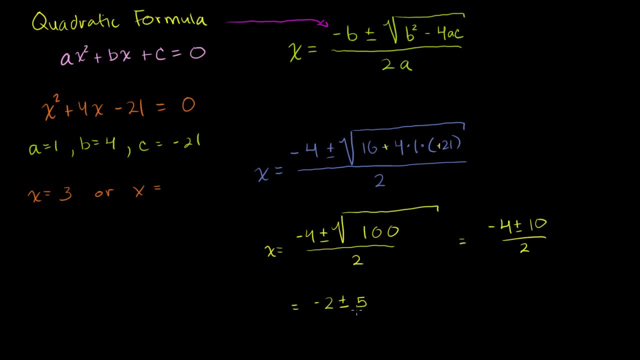 which is 3, or x, could be equal to negative 2 minus 5,, which is negative 7.. So the quadratic formula seems to have given us an answer for this. You can verify just by substituting back in that these do work. 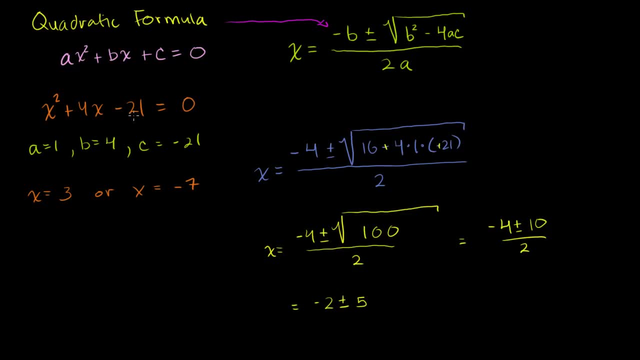 Or you could even just try to factor this right here: You say: what two numbers. when you take their product, you get negative 21. And when you take their sum, you get positive 4. So you'd get x plus 7 times x minus 3 is equal to negative 21.. 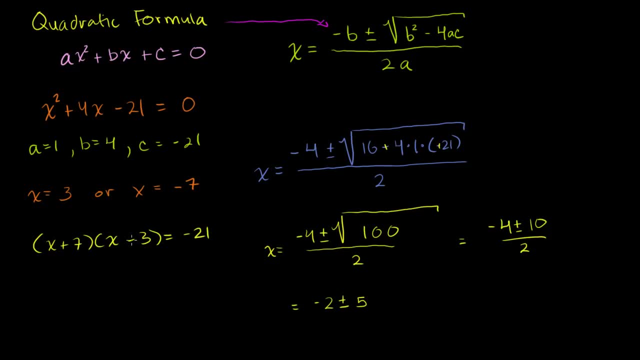 Notice: 7 times negative, 3 is negative 21.. 7 minus 3 is positive 4. You would get x plus- sorry, it's not negative 21, is equal to 0. There should be a 0 there. 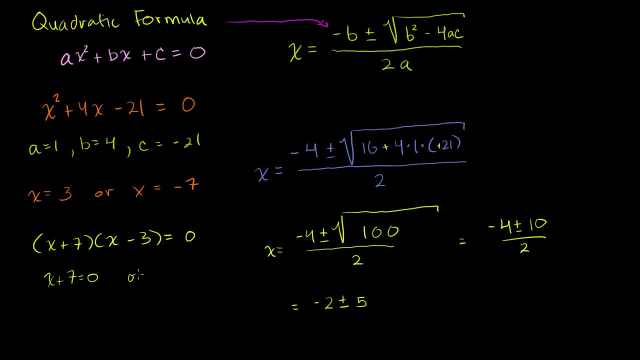 So you'd get x plus 7.. You'd get x plus 7 is equal to 0, or x minus 3 is equal to 0.. x could be equal to negative 7, or x could be equal to 3.. 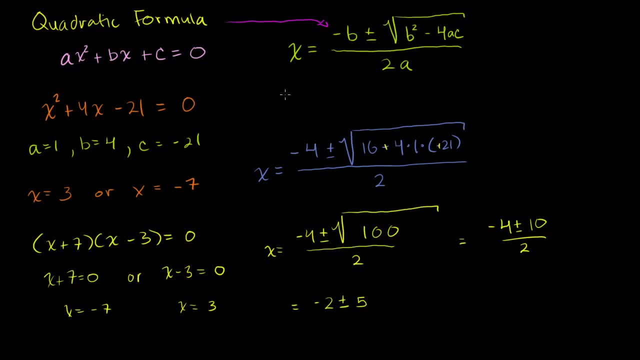 So it definitely gives us the same answer as factoring. So you might say, hey, why bother with this crazy mess? And the reason we want to bother with this crazy mess is it'll also work for problems that are hard to factor, And let's do a couple of those. 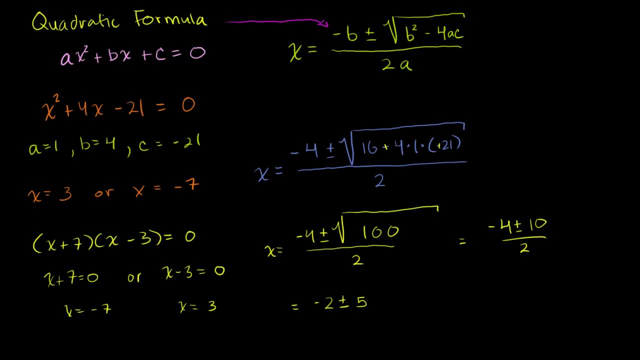 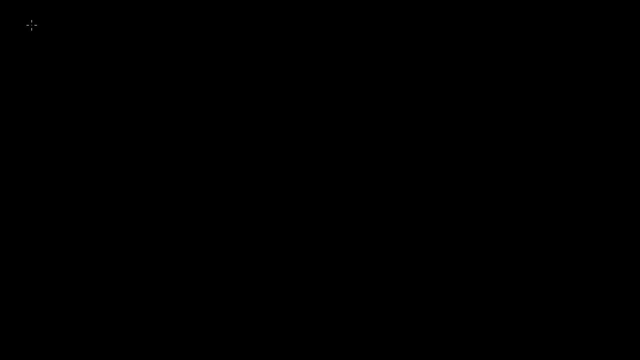 Let's do some hard to factor problems right now. Scroll down, get some fresh real estate. Let's rewrite the formula again, just so we have, in case we haven't had it memorized yet. x is going to be equal to negative, b plus or minus. 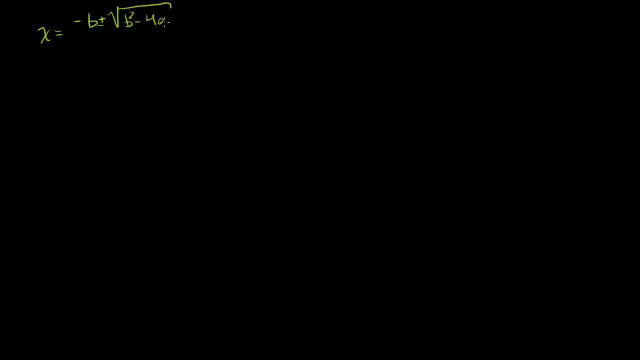 the square root of b squared minus 4ac. all of that over 2a. Now let's apply this to another problem. Let's say we have the equation 3x squared plus 6x is equal to negative 10.. 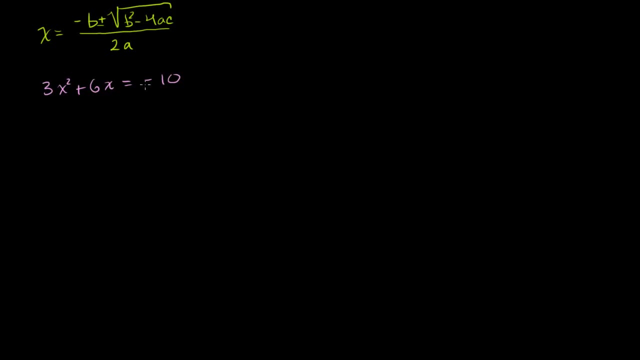 Well, the first thing we want to do is get it in the form where all of our terms are on the left-hand side. So let's add 10 to both sides of this equation. We get 3x squared plus 6x plus 10 is equal to 0.. 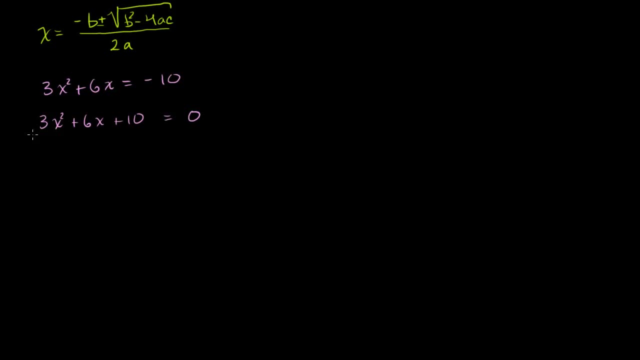 And now we can use the quadratic formula, So let's apply it here. So a is equal to 3.. That is a, This is b And this right there is c. So the quadratic formula tells us the solutions to this equation, the roots of this quadratic function. 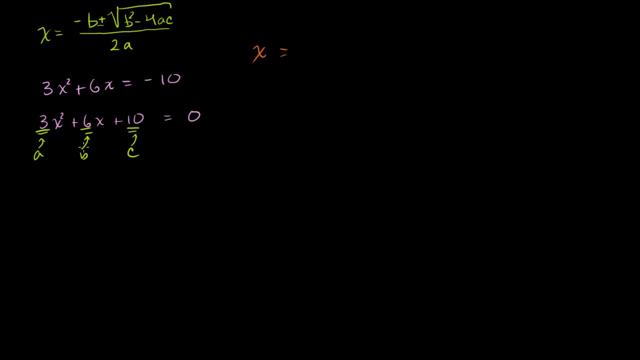 I guess we could call it: x is going to be equal to negative b. Negative b b is 6.. So negative 6 plus or minus. the square root of b squared b is 6.. So we get 6 squared. 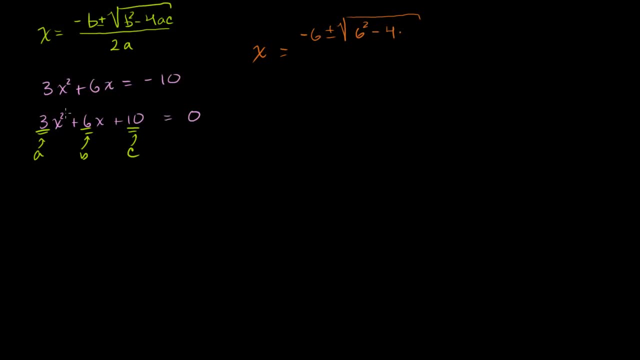 b squared minus 4 times a, which is 3, times c, which is 10.. Stretch out the radical a little bit: All of that over 2 times a, 2 times a, 2 times 3.. So we get: x is equal to negative, 6 plus or minus the square root. 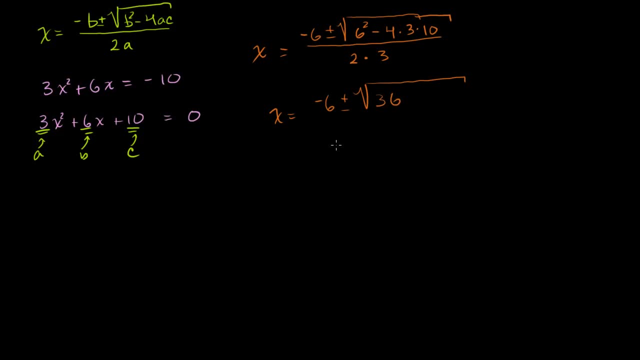 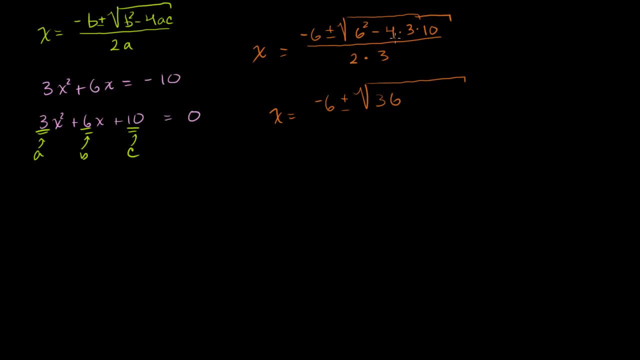 36. This is interesting. Minus 4 times 3 times 10.. So this is minus, Let me make sure. Yeah, 4 times 3 times 10 is minus 120.. Minus 120.. All of that over 6.. 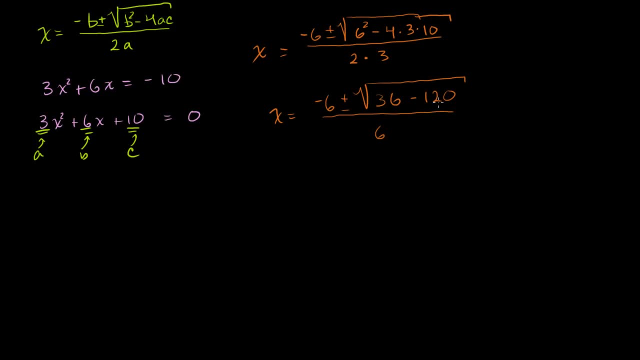 So this is interesting. You might already realize why it's interesting. What is this going to simplify to? That's 84 if I'm doing my 120 minus 36.. We make this into a 10, then this will become an 11.. 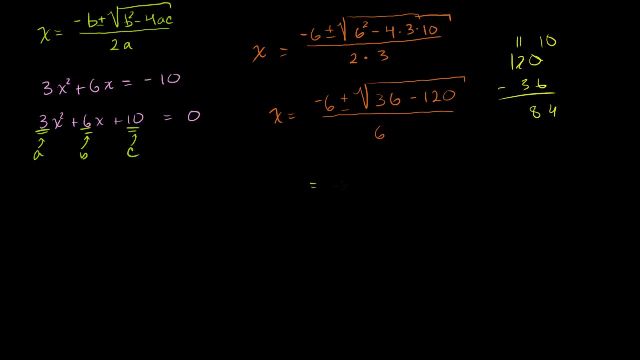 This is a 4. It is 84. So this is going to be equal to negative 6 plus or minus the square root of, but not positive, 84. That's, if it's 120 minus 36. We have 36 minus 120.. 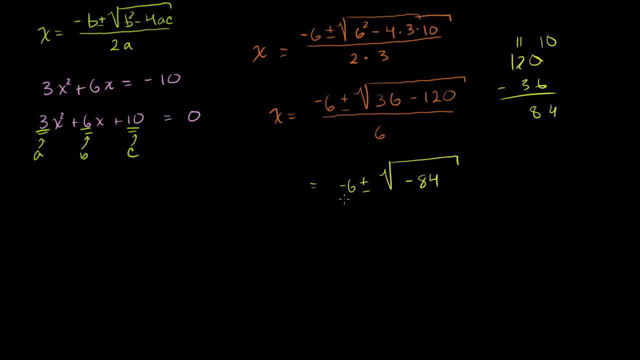 It's going to be negative 84.. All of that over 6.. So you might say, gee, this is crazy. What is this silly quadratic formula you're introducing me to Sal? It's worthless. It just gave me a square root of a negative number. 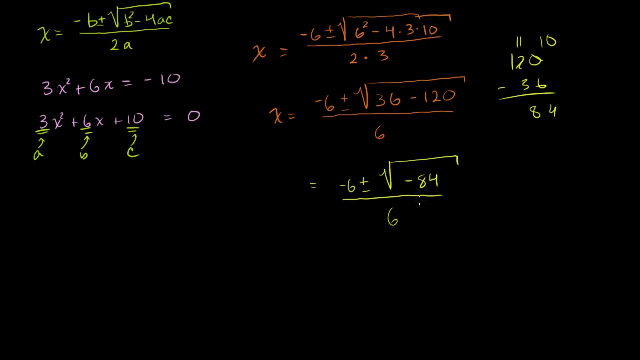 It's not giving me an answer, And the reason why it's not giving you an answer, or at least an answer that you might want, is because this will have no real solutions In the future. we're going to introduce something called an 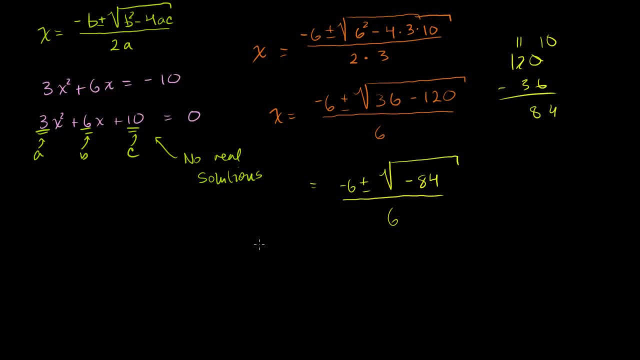 imaginary solution. We're going to take an imaginary number which is a square root of a negative number and then we can actually express this in terms of those numbers. So this actually does have solutions, but they involve imaginary numbers, So this actually has no real solution. 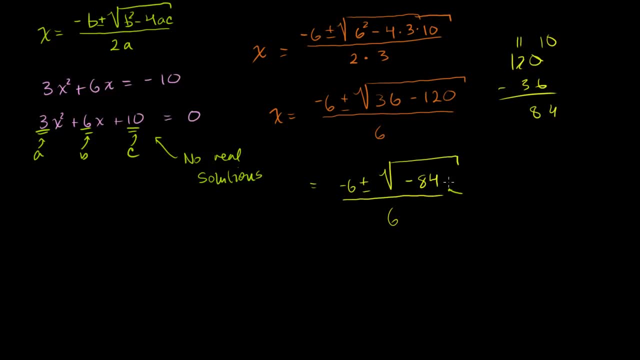 We're taking a square root of a negative number, So the b squared with the b squared minus 4ac. if this term right here is negative, then you're not going to have any real solutions, And let's verify that for ourselves. 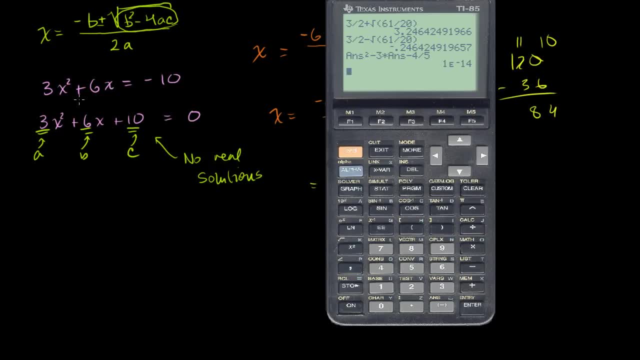 Let's get our graphing calculator out And let's graph this equation right here. So let's get the graph. y is equal to- that's what I had there before- 3x squared plus 6x plus 10.. So that's the equation. 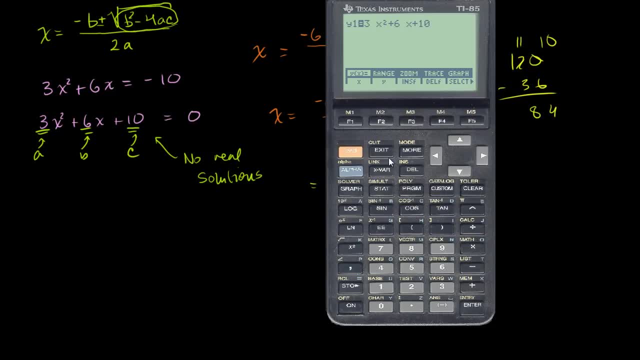 We're going to see where it intersects the x-axis. Where does it equal 0?? So let me graph it. Notice: this thing just comes down and then goes back up. Its vertex is sitting here above the x-axis and it's 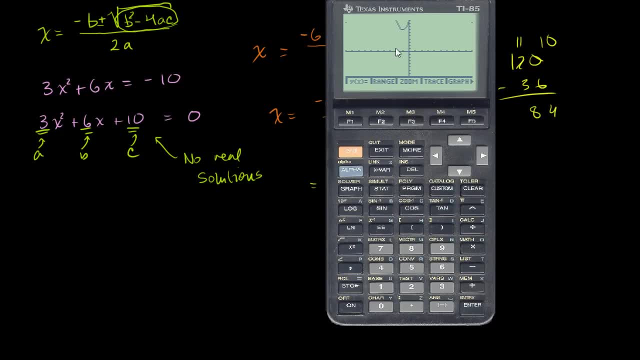 upward opening. It never intersects the x-axis. So at no point will this expression, will this function equal 0.. At no point will y equal 0 on this graph. So once again, the quadratic formula seems to be working. Let's do one more example. 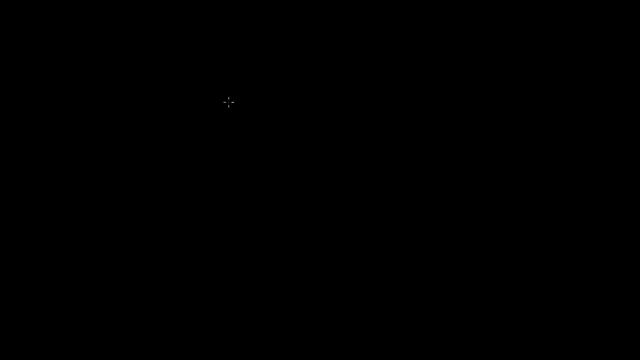 You can never see enough examples here And I want to do ones that are maybe not so accurate, So obvious to factor. So let's say we get negative: 3x squared plus 12x plus 1 is equal to 0.. Now let's try to do it just having the quadratic formula. 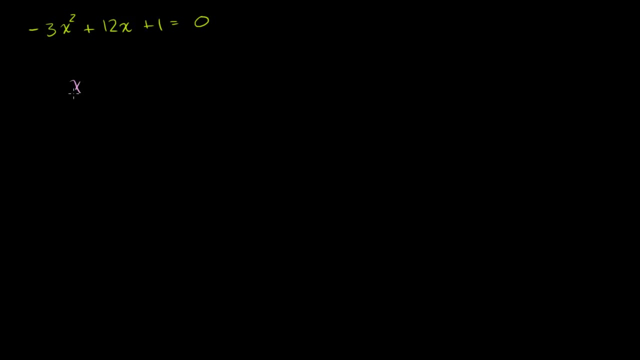 in our brain. So the x's that satisfy this equation are going to be negative b. This is b, So negative b is negative 12 plus or minus the square root of b squared of 144.. That's b squared minus 4 times a, which is negative 3, times. 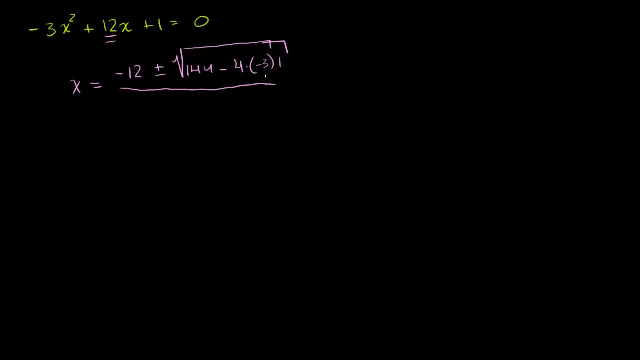 c, which is: 1. All of that over 2 times a, over 2 times negative 3. So all of that over negative 6. This is going to be equal to negative 12 plus or minus. the square root of what is this: 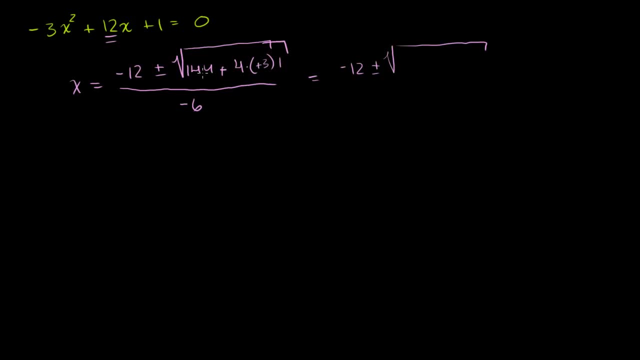 The negative times. a negative they cancel out. So I have 144 plus 12.. So that is 156.. 144 plus 12.. All of that over negative 6.. Now I suspect we can simplify this 156.. We can maybe bring some things out of the radical sign. 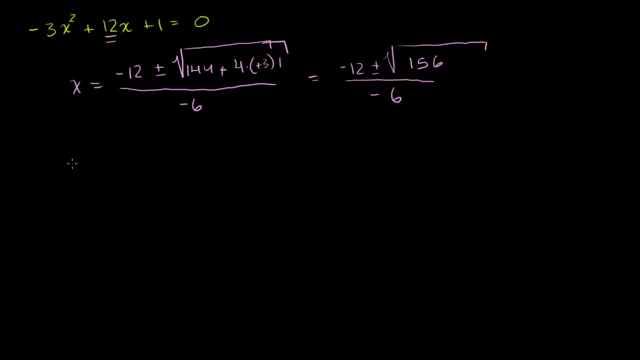 So let's attempt to do that. So let's do a prime factorization of 156.. Sometimes this is the hardest part: simplifying the radical. So 156 is the same thing as 2 times 78.. 78 is the same thing as 2 times what? 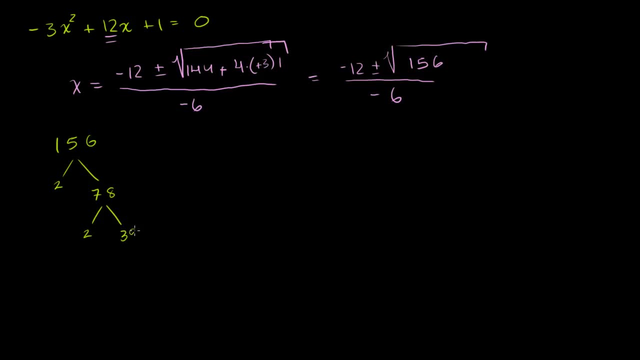 That's 2 times 39. So the square root of 156 is equal to the square root of 2 times 2.. 2 times 39. Or we could say: that's the square root of 2 times 2 times the square root of 39.. 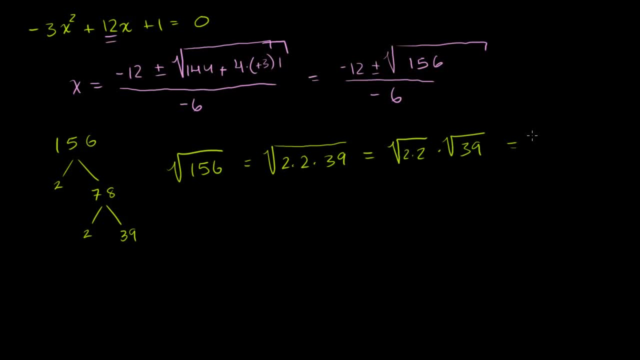 And this, obviously, is just going to be the square root of 4, or this is the square root of 2 times 2.. It's just 2.. 2 square roots of 39, if I did that properly, Let's see 4 times 39.. 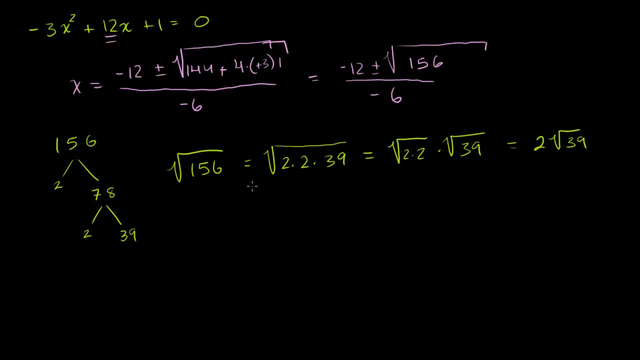 Yeah, it looks like it's right: 120.. Yep, So this up here will simplify to negative 12 plus or minus 2 times the square root of 39.. 39.. All of that over negative 6.. Now we can divide the numerator and the denominator by 2.. 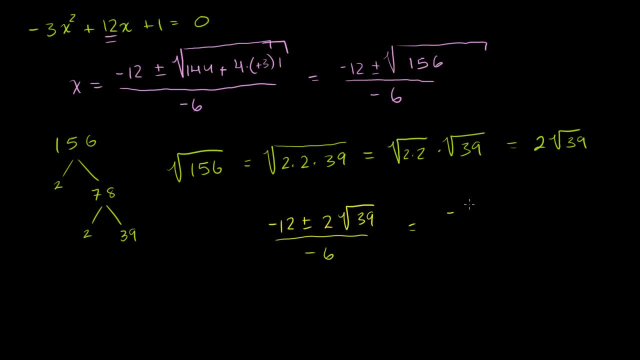 So this will be equal to negative 6 plus or minus the square root of 39 over negative 3.. Or we could separate these two terms out. We could say this is equal to negative 6 over negative 3 plus or minus the square root of 39 over negative 3.. 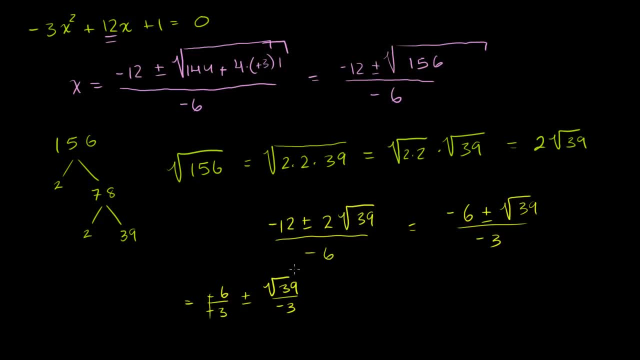 Now, this is just a 2, right here. right, These cancel out. 6 divided by 3 is 2.. So we get 2.. And now notice: if this is plus and we use this minus sign, the plus will become negative and the negative. 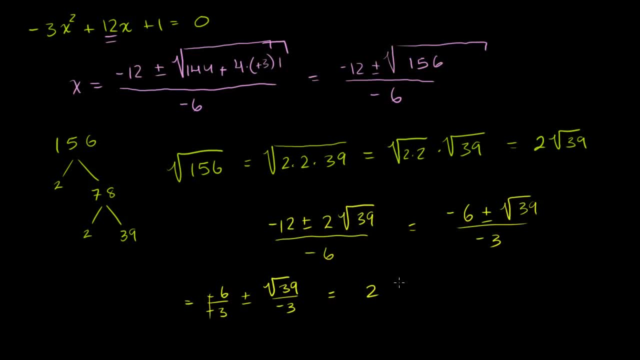 will become positive, But it still doesn't matter, right? We could say minus or plus, or that's the same thing as plus or minus, the square root of 39 over 3.. I think that's about as simple as we can get this answer. 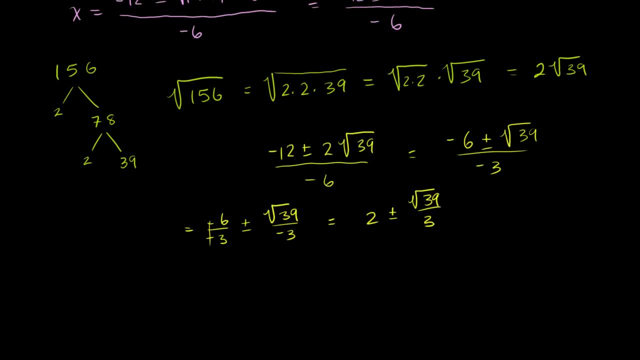 Now I want to make a very clear point of what I did at that last step. I did not forget about this negative sign. I just said it doesn't matter, It's going to turn the positive into the negative. It's going to turn the negative into the positive. 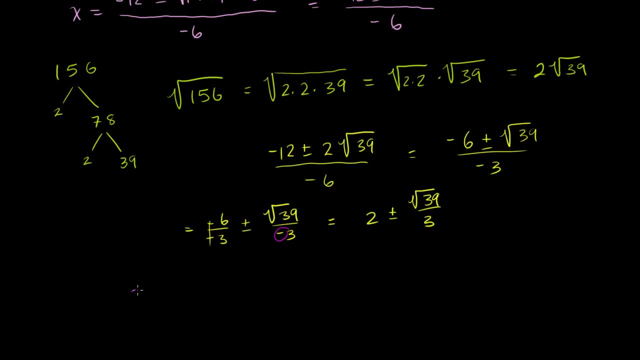 Let me rewrite this, So this right here can be rewritten as 2 plus the square root of 39 over negative 3, or 2 minus the square root of 39 over negative 3, right, That's what the plus or minus means. 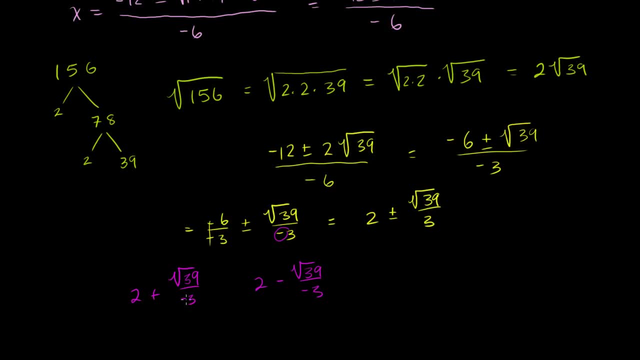 It could be this or that or both of them. really, Now, in this situation, this negative 3 will turn into 2 minus the square root of 39 over 3, right, I'm just taking this negative out Here, the negative and the negative will become a. 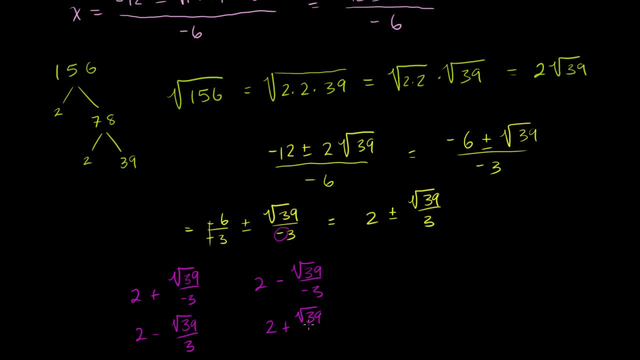 positive and you get 2 plus the square root of 39 over 3, right negative times, a negative is a positive. So once again you have 2 plus or minus the square root of 39 over 3.. 2 plus or minus the square root of 39 over 3 are solutions to. 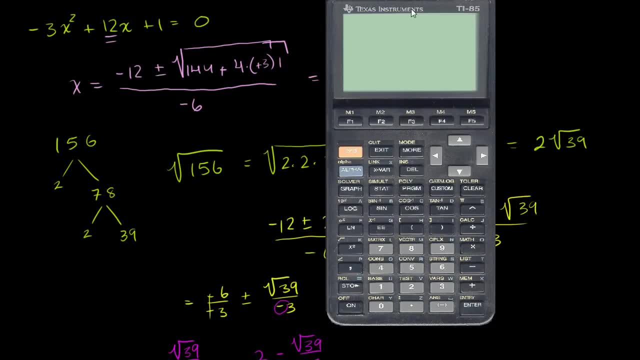 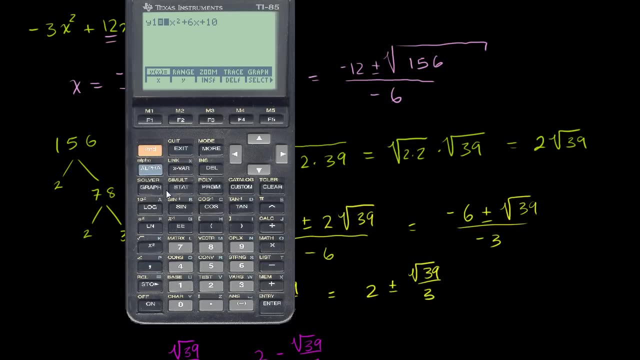 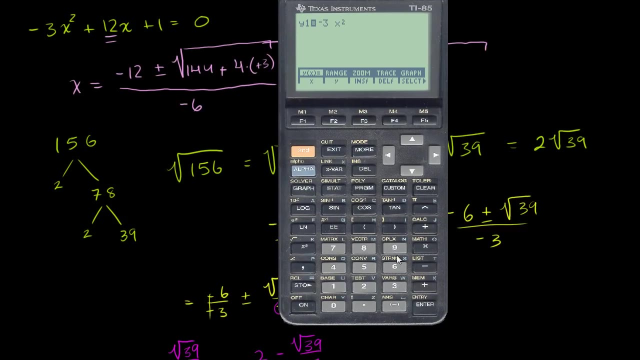 this equation right there, Let's verify. I'm just curious what the graph looks like, So let's just look at it. So let me clear this: Where's the clear button? So we have negative 3x squared plus 12x plus 1.. 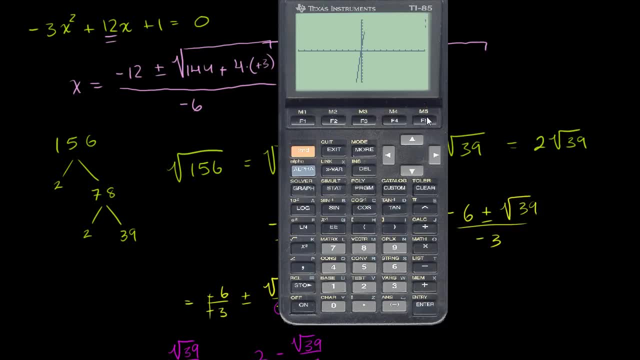 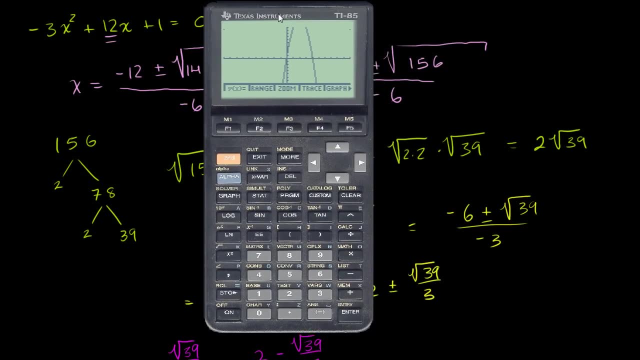 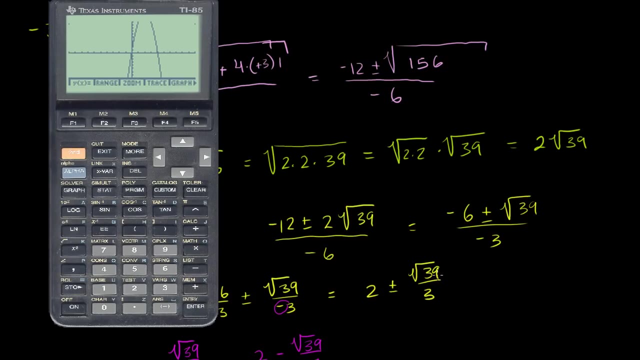 And let's graph it. Let's see where it intersects the x-axis. It goes up there and then back down again. So 2 plus or minus the square root- See the square root of 39- is going to be a little bit more. 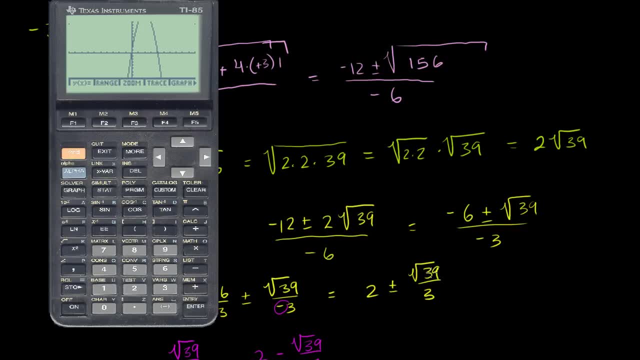 than 6, right, Because 36 is 6 squared, So it's going to be a little bit more than 6.. So this is going to be a little bit more than 2.. A little bit more than 6 divided by 3 is a little bit. 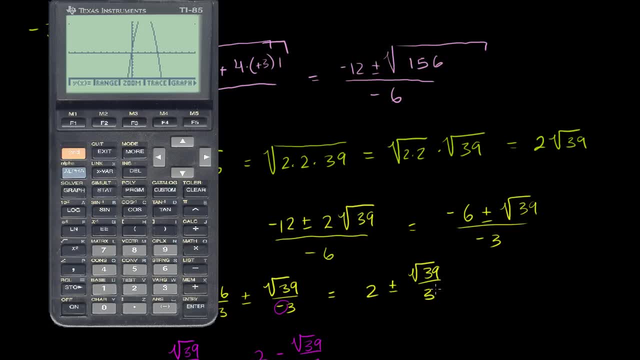 more than 2.. So you're going to get one value that's a little bit more than 4, and then another value that should be a little bit less than 1.. And that looks like the case You have 1,, 2,, 3,, 4.. 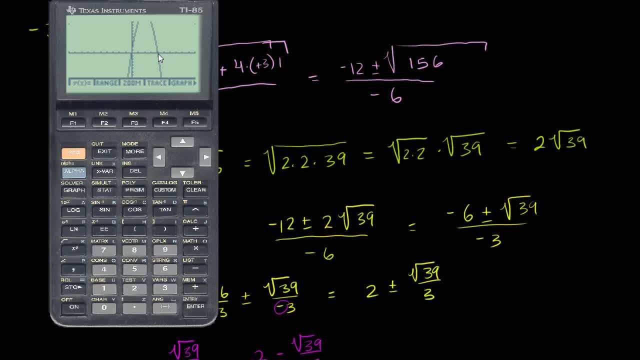 You have a value that's pretty close to 4, and then you have another value that is a little bit. maybe it looks close to 0, but a little bit less than that. So anyway, hopefully you found this application of the quadratic formula helpful.